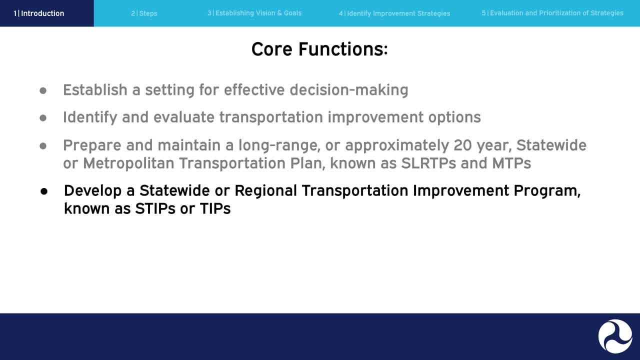 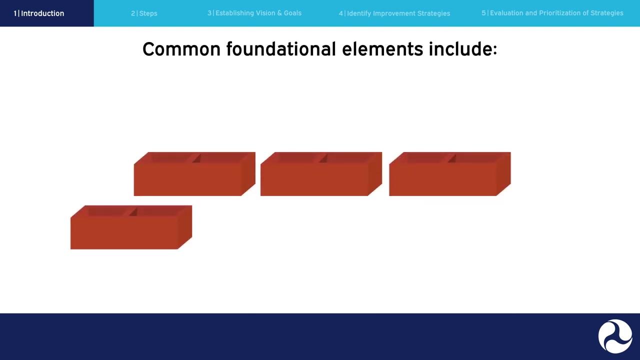 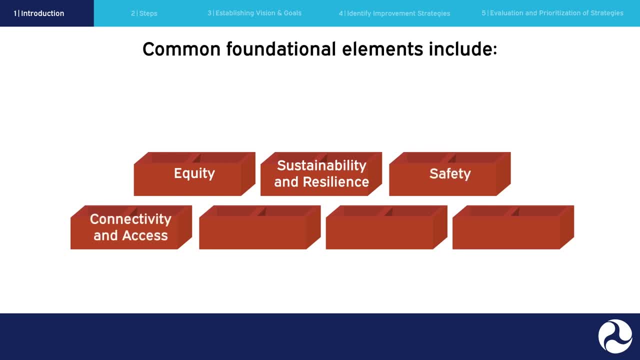 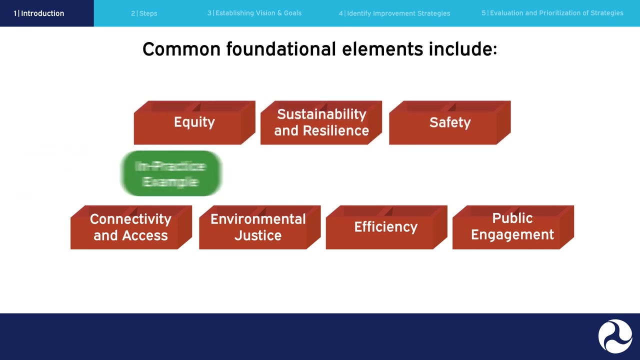 resilience, safety, connectivity and access, environmental justice, efficiency and public engagement. All planning activities should take these issues into consideration and incorporate them into the planning process. As we progress, we will highlight these issues within each step of the planning process, Additionally using an in-practice example. we will follow the course. 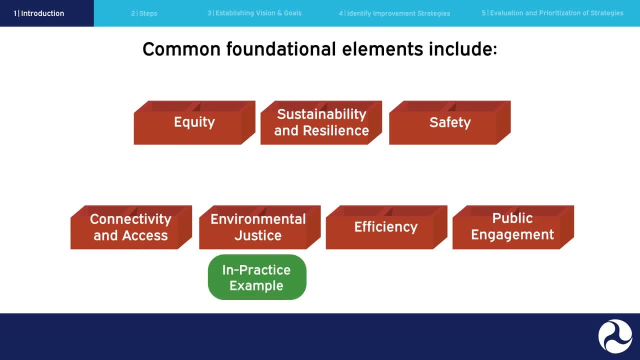 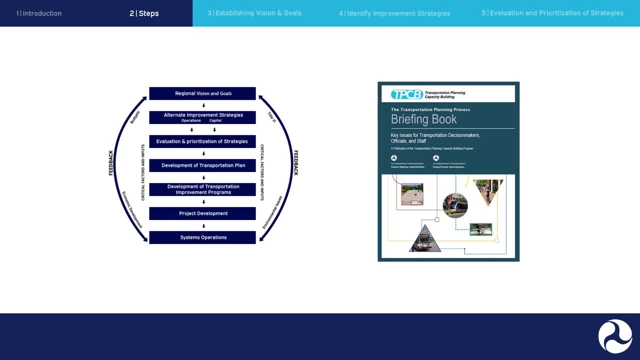 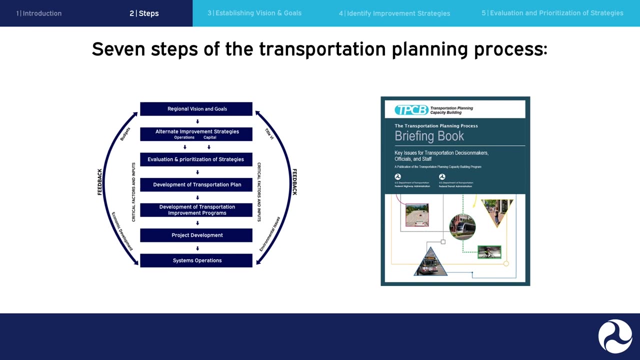 of a hypothetical project as it moves through each step of the transportation planning process, Steps From the briefing book and the graphic shown earlier. we are using these seven steps to illustrate the transportation planning process. Keep in mind that, to accommodate the complex realities of the real world, the process is often less straightforward than is presented here. 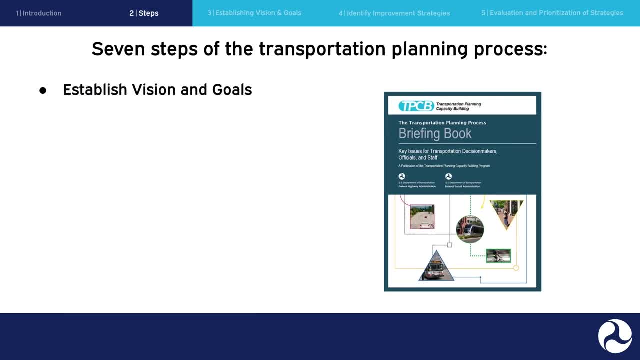 The seven steps are: establish vision and goals, identify improvement strategies, evaluate and prioritize strategies, develop a transportation plan, develop a transportation improvement program, implement the transportation plan and operate the system. Let's go through each of these steps one by one at the MPO level: Establishing vision and goals. 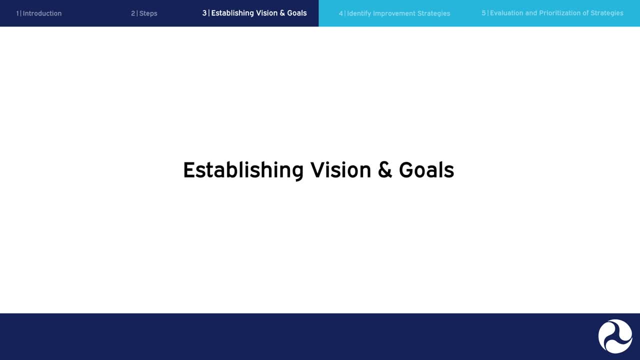 The first step in the transportation planning process is to define your vision and your goals. An example of a community's vision is what members of that community might want it to look like in the next 20 years. while goal statements address specific issues and aspirations, The vision and goals will vary depending on your organization, your location. 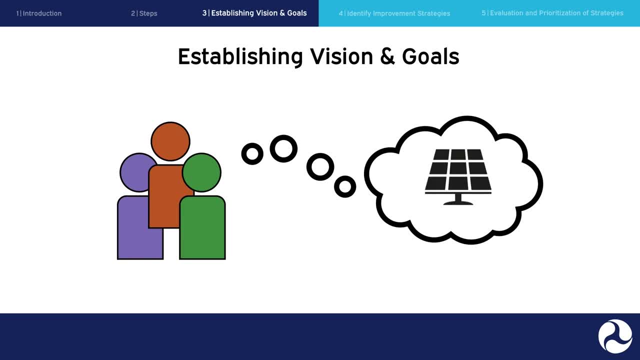 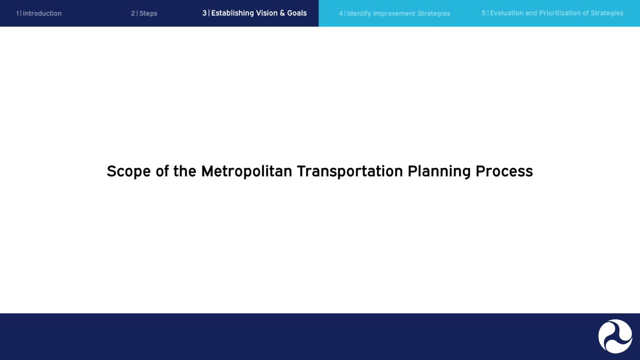 and the needs of the community. While every community's vision and goals may differ from one another, the process of establishing them can be similar. When establishing your vision and goals, planning organizations should address certain established planning factors already listed on their website, To incorporate that to your Logo. 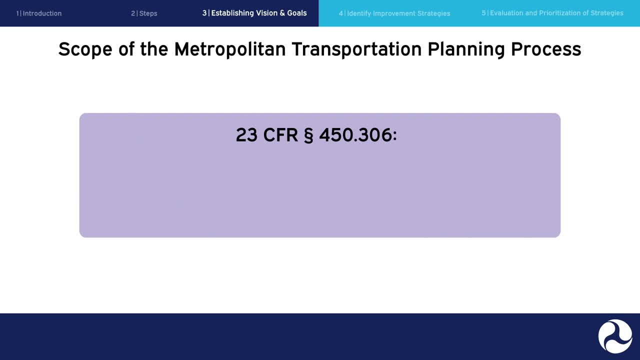 you must set up a report, graphic article or assessment resource Scope of the Metropolitan Transportation Planning Process. That regulation states that the Metropolitan Transportation Planning process shall be continuous, cooperative and comprehensive and provide for consideration and implementation of projects, strategies and services that will address the following factors: Support the economic vitality of the metropolitan. area. Increase the safety of projects and services�. challenge and services. increase various aspects of the metropolitan area and theirbrush aspects of the metropolitan area. RE thee task: concept of sacrificing practices, including administrative and administrative phases for którą bi 이해, the citizens assault, and Venus logistics responsibilities. 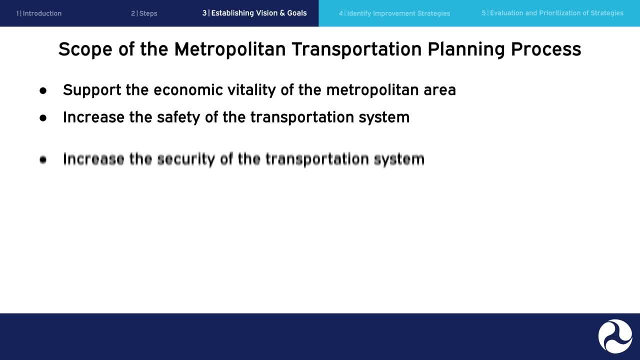 Derivate a measurement protocol for exchange, evacuation and monetary maintenance of the facilities. It requires all religious empires andilleurs and everyone's requirements. Thisあと ella: safety of the transportation system. increase the security of the transportation system. 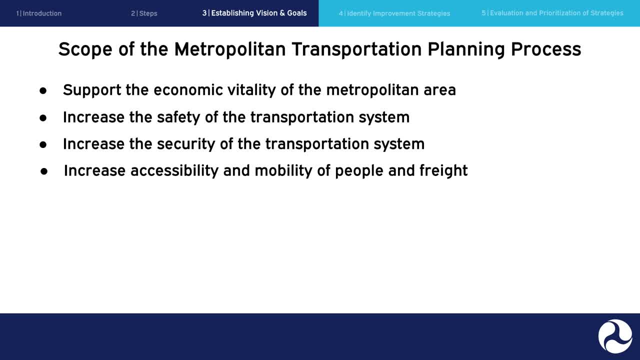 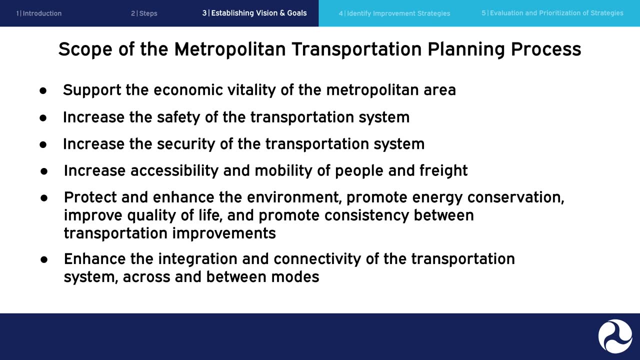 increase accessibility and mobility of people and freight, protect and enhance the environment, promote energy conservation, improve quality of life and promote consistency between transportation improvements enhance the integration and connectivity of the transportation system across and between modes, promote efficient system management and operation. 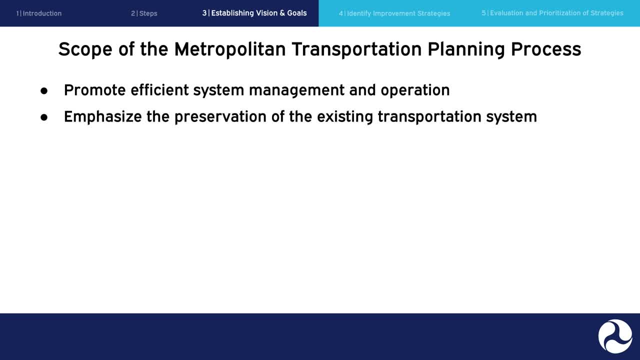 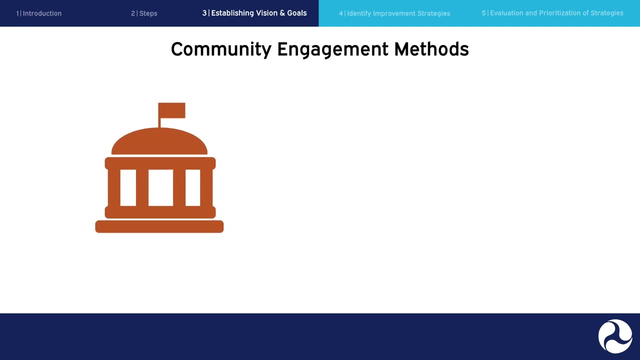 emphasize the preservation of the existing transportation system, improve the resiliency and reliability of the transportation system, and enhance travel and tourism. When establishing your vision and goals, community engagement is key. Your organization should conduct outreach across communities in your areas, ensuring that all voices are heard. 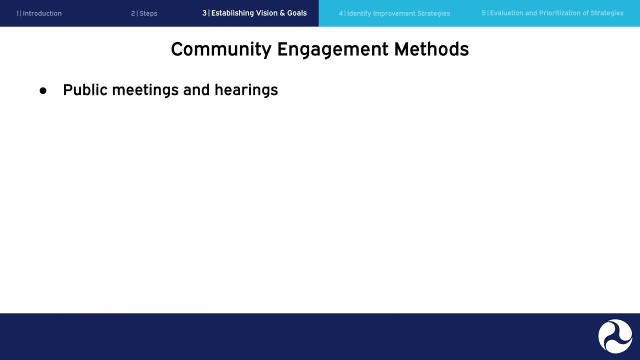 There are many engagement methods, including public meetings and hearings, workshops, charrettes and town halls, social media outreach, engagement with community groups and local organizations, pop-up outreach and virtual public involvement. For more information on FHWA's virtual public involvement initiative, see the FHWA's VPI website. 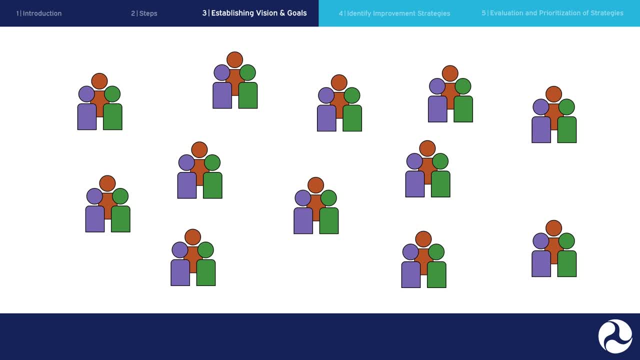 These are just a few of the methods that can be used, and an effective community engagement strategy should employ multiple methods. It is imperative that communities whose voices are often not heard within planning processes are engaged in meaningful ways. These communities may include those with limited English proficiency. 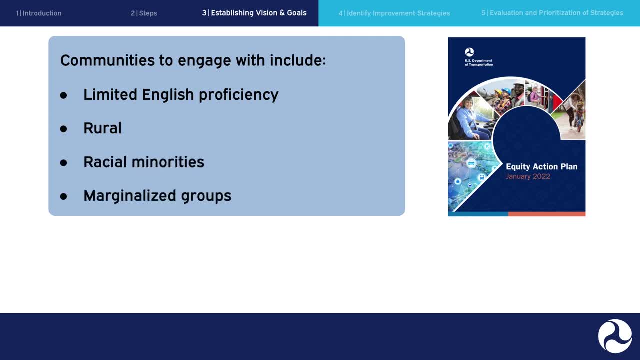 rural communities, racial minorities and other marginalized groups. For more information on conducting equitable public outreach, see the FHWA's site on Environmental Justice in the USDOT Equity Action Plan. Let's look at the Plannersburg NPO's up-to-date plan to help award students who have a policy. 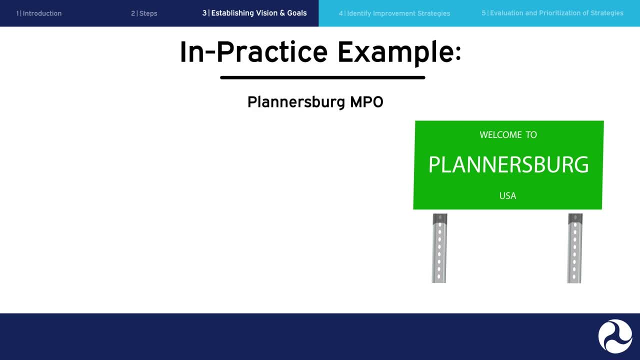 experience and perform well in the field of public policy on environmental justice. For our in-practice example, let's look at the Plannersburg MPA's Entry Grant Program. Let's look at the Plannersburg MPO, which is a single-county MPO consisting of the city of 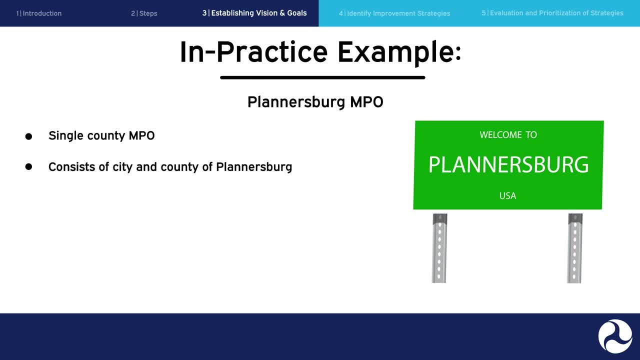 Plannersburg and the county of Plannersburg. The MPO is working with the city to update their vision for their transportation system. Plannersburg MPO and city staff begin a public engagement process reaching out to communities throughout their city. Through this engagement, they identify: 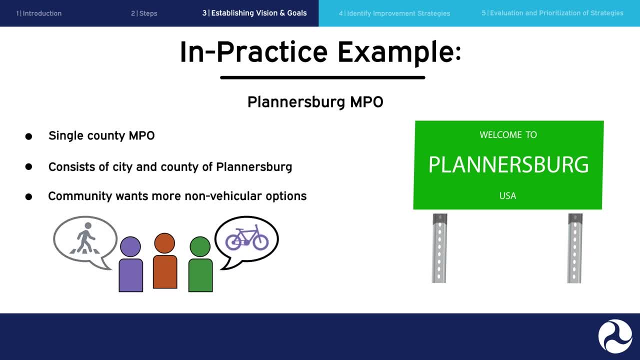 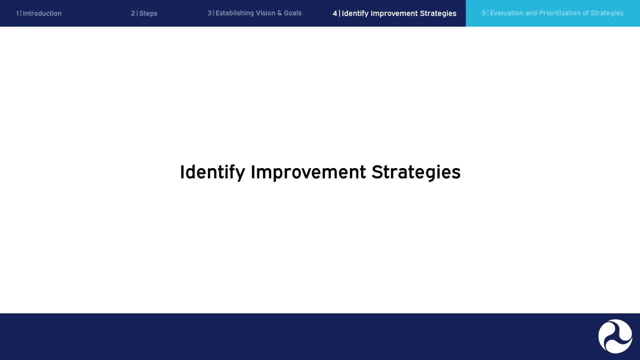 that community members desire a wider array of non-vehicular transportation options that connect all parts of the city. They establish a goal to build connections via more sustainable transportation options. Identify improvement strategies. In this next step, your organization will build upon the vision and goals developed in the previous step to identify the needs and 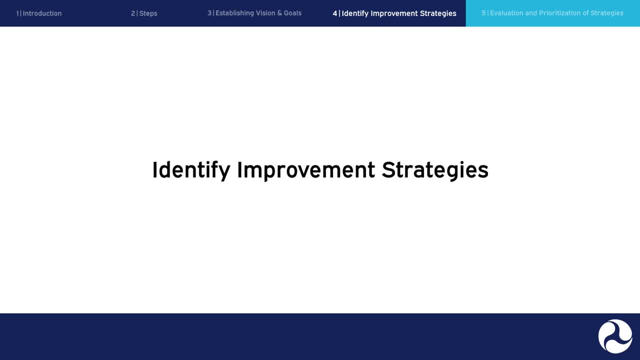 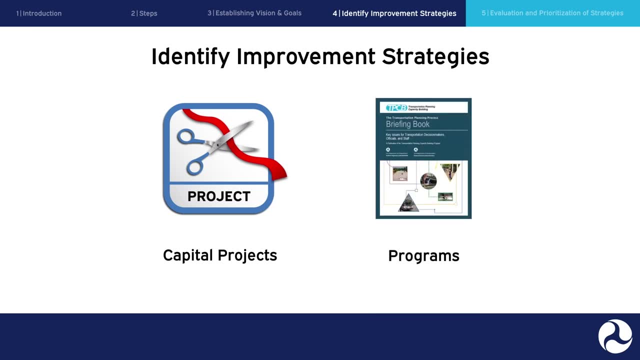 gaps that can be addressed through various strategies. These strategies may be capital projects like adding a roundabout, or a program like developing complete streets, policies or guidance for local agencies. You will compare the vision and goals against existing and future conditions within the planning area to identify possible strategies that are responsive. 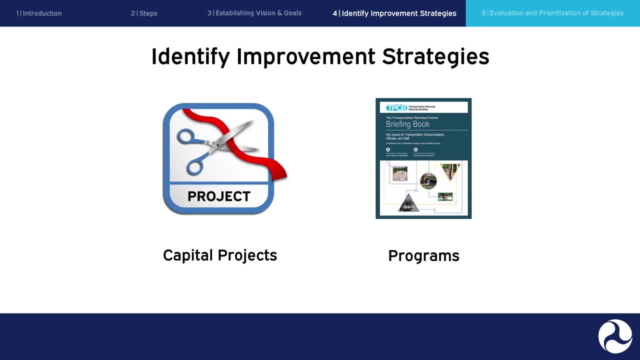 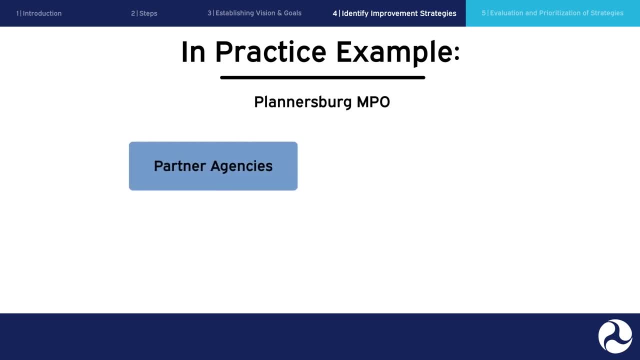 to current conditions and will continue to be relevant into the future. In Practice Example, The MPO staff work with partner agencies synthesize the result from the previous community engagement, their analysis of the planning area's existing conditions and their understanding of the existing conditions. There are different strategies to identify. 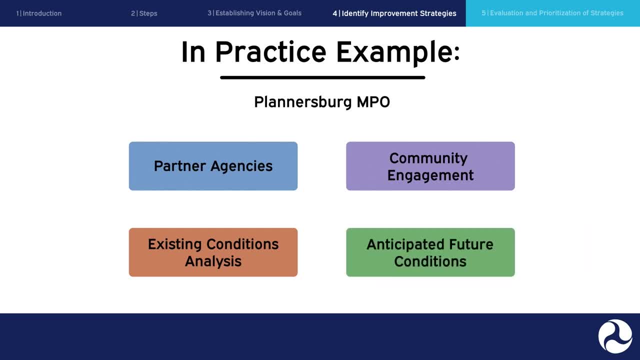 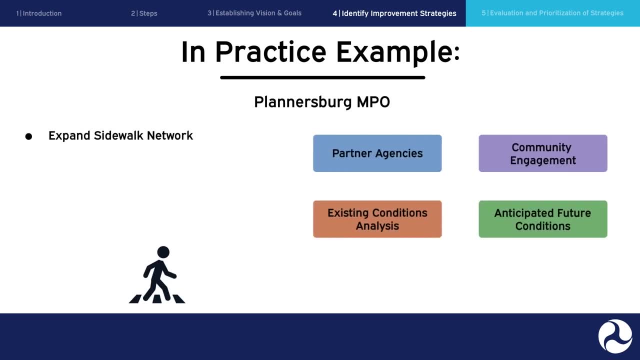 of anticipated future conditions to identify a range of non-vehicular strategies that would improve connectivity. The MPO recommends strategies to expand the sidewalk network, construct bike lanes and additional bicycle infrastructure, expand the bus surface and add e-scooter and bike share services. Evaluation and Prioritization of Strategies. 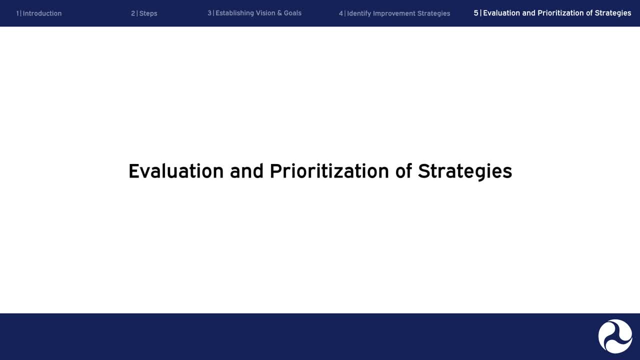 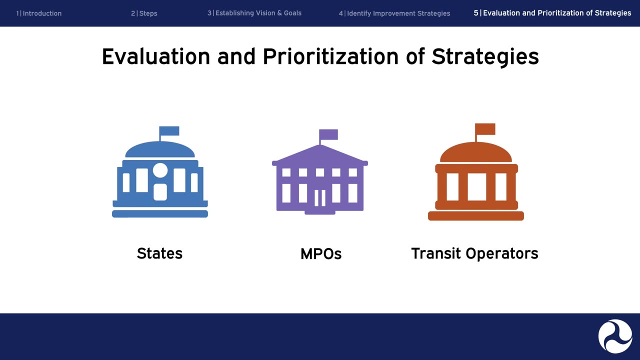 After identifying improvement options, those strategies must then be evaluated and prioritized to align with available resources and community interests. Prioritization is a cooperative process among states, MPOs and transit operators for identifying projects and strategies from the most recent 20-year Long-Range Metropolitan Transportation Plan, or MTP, that are 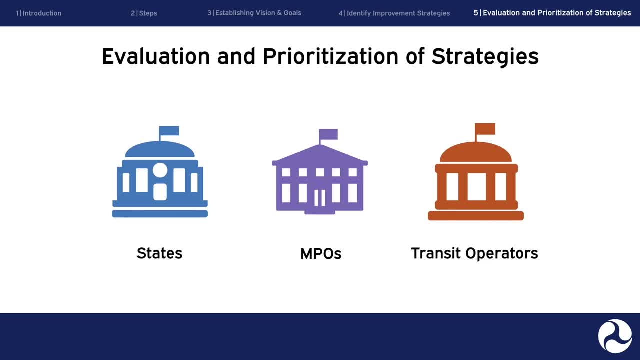 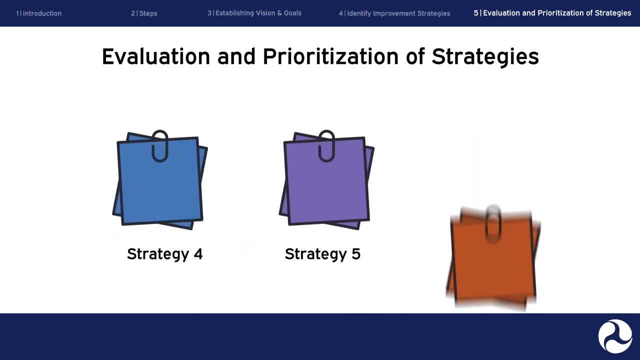 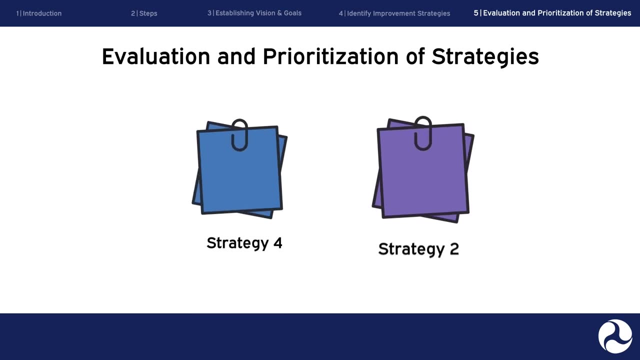 sufficiently high priority and ready for delivery to be included in the TIP? What strategies will best align with your organization's vision or goals? What strategies will be the most popular or impactful to your community? What strategies are the most cost-effective or efficient? These are some of the questions you 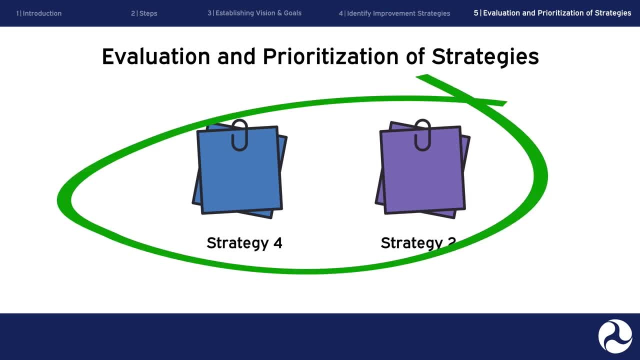 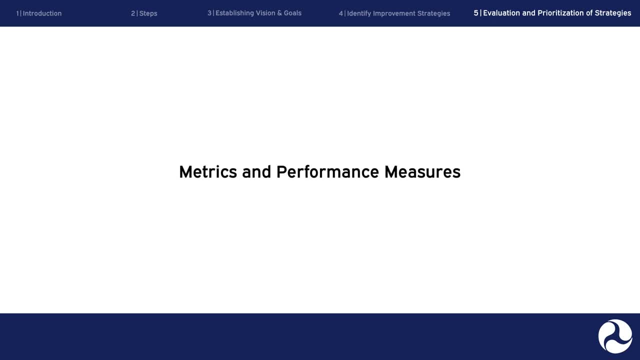 will be asking yourself as you move through this process. To answer those questions, you will evaluate the strategies via a defined set of metrics and performance measures. These metrics will vary across locations and agencies, but commonly include mobility, equity, environmental justice, access, safety, sustainability, connectivity. 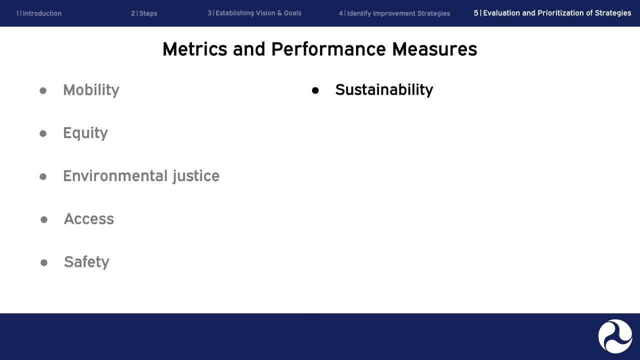 cost-benefit or alignment with existing plans, laws and state and federal guidance. When you are going through the prioritization process, you will want to continue engaging the public. Be sure to follow your public participation plan and pay particular attention to seek fairness in meeting the needs of all community members, including people studying. 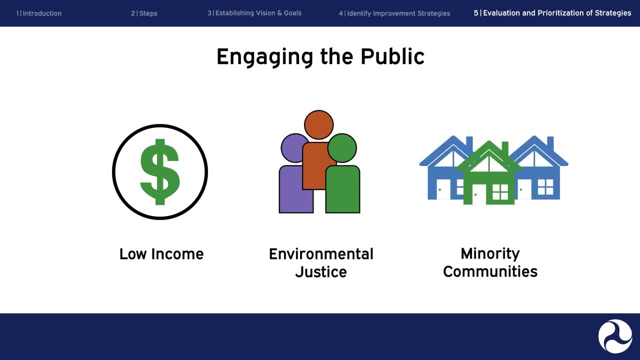 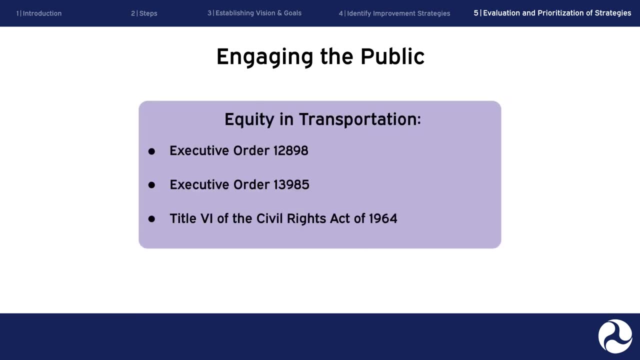 low-income, environmental, justice and minority communities, who have often been overlooked in past transportation planning processes. It is crucial that you engage previously overlooked communities when prioritizing strategies. There are a number of executive orders, as well as the Civil Rights Act of 1964, which can help you address these issues. For more information, 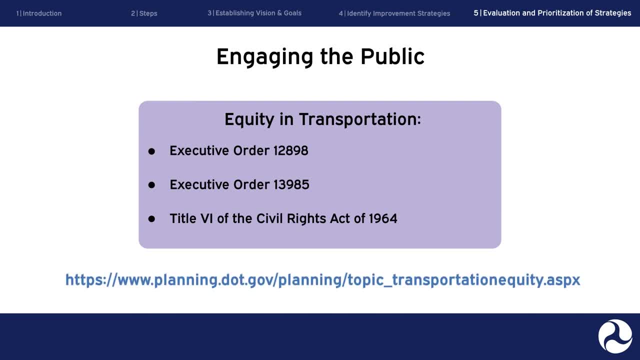 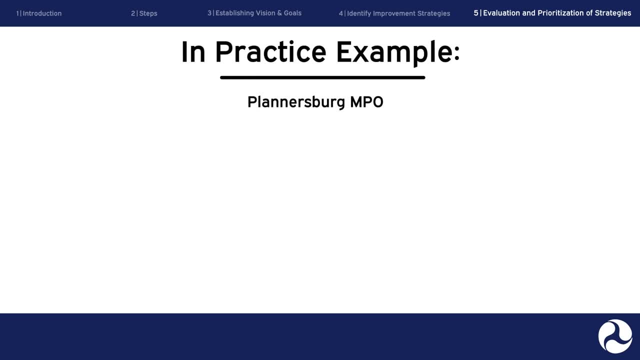 see the USDOT webpage on transportation equity In practice. example: staff for the Plannersburg MPO convene a committee of representatives from local agencies, the state, DOT and environmental and economic development organizations to prioritize the strategies that they previously developed through the planning process. The committee applies the evaluation criteria that 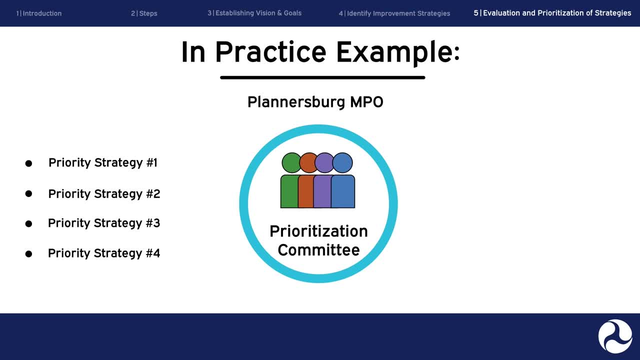 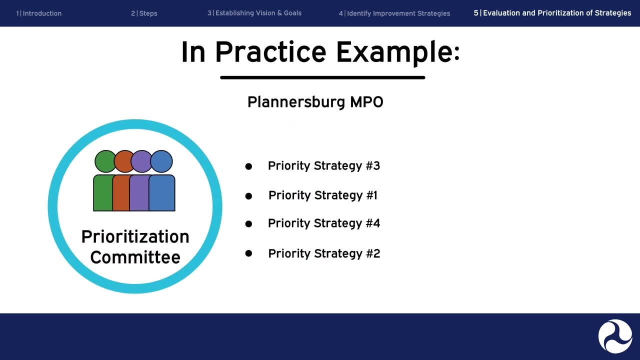 were developed in advance and aligned with the goals of the MTP. They evaluate benefits, trade-offs, costs, liabilities, project readiness and community engagement responses, including outreach to marginalized communities. They then rank strategies to align with available resources. These recommendations are presented to the MPO Policy Committee that will ultimately decide. 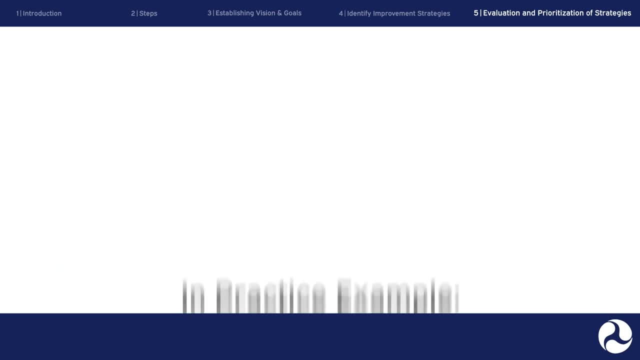 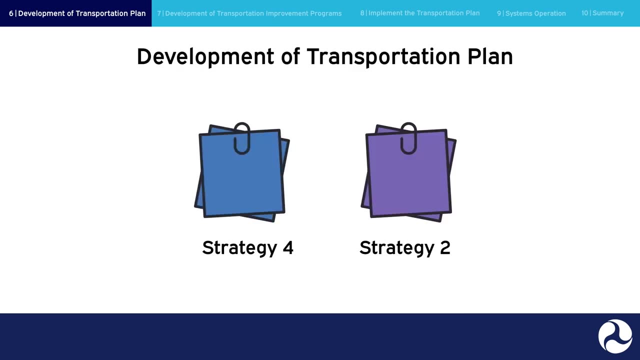 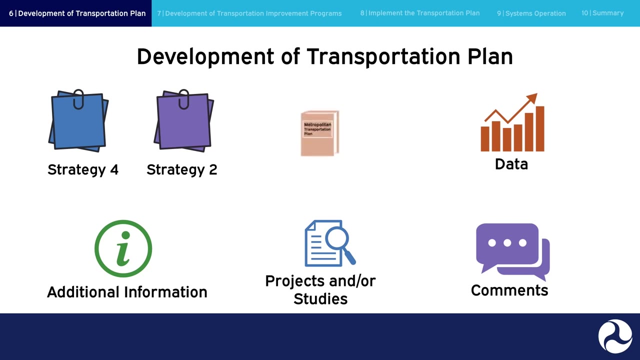 what strategies to include in the plan. Development of Transportation Plan. Once strategies are evaluated and prioritized, they are combined with additional information, data, comments, projects and or studies into the Metropolitan Transportation Plan. This plan may incorporate additional public comments. peer agency input. 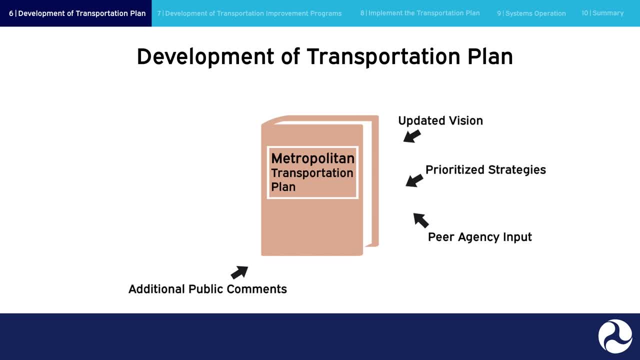 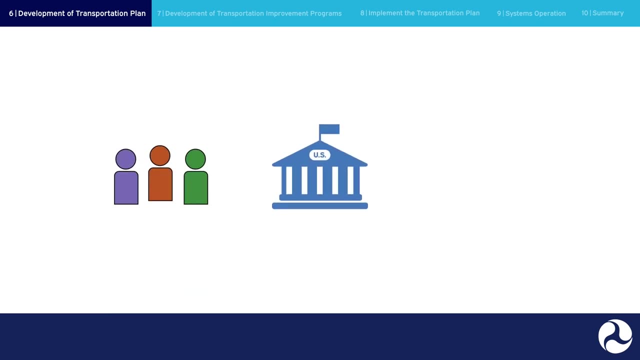 prioritized strategies, an updated vision and air quality analysis. The plan will include detailed information on capital projects, proposed policies, operational strategies and funding mechanisms. This process has many steps itself Along the way. there are a range of projects that will be included in the plan. There are a number of projects that 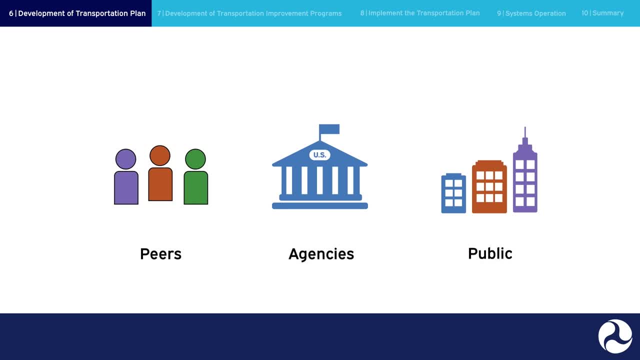 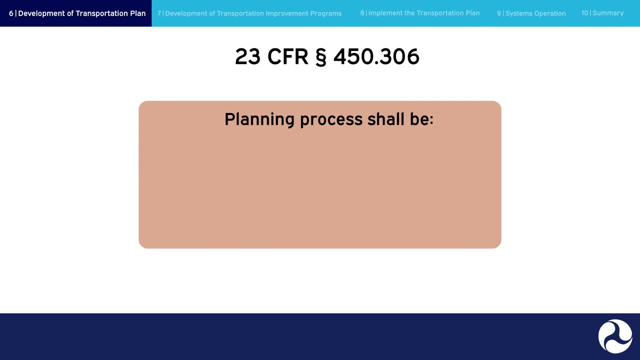 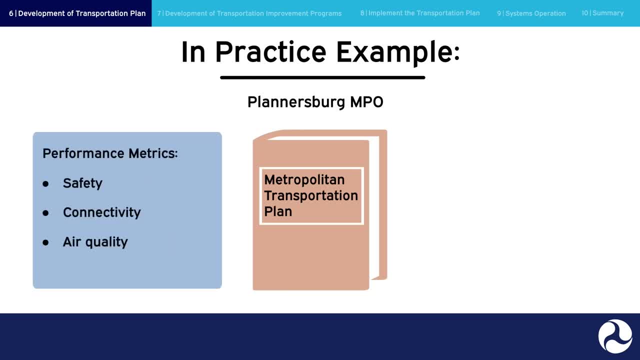 intended to measure safety, connectivity and air quality, among other factors. This document provides a long-range vision for the planning area and lays out the vision, goals, strategies and priorities. It also defines performance measures, as well as project program and policy recommendations. Within the plan, complete street strategies are prioritized. 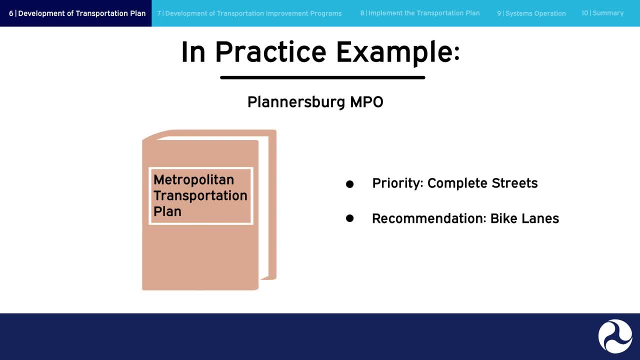 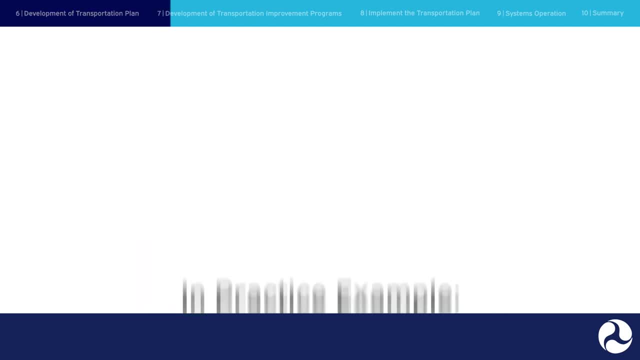 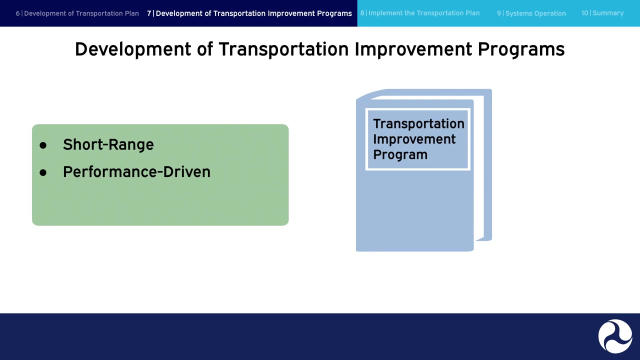 and bike lanes are highlighted as a project recommendation. General information, including potential location and broad design guidance, is included. Development of Transportation Improvement Programs: From the longer-term, larger-scale transportation plan that you developed in the previous step, a short-range, performance-driven transportation improvement program is developed that includes: 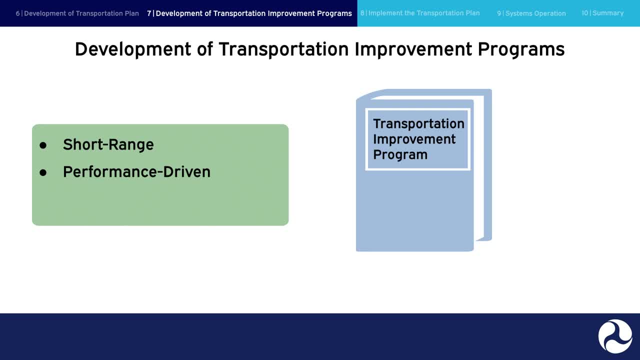 priority transportation improvements. The TIP implements the long-range transportation plan. Programs include funding for projects over a four-year period. The TIP at the MPO level or STIP at the statewide level represents immediate priority actions to achieve the area's goals and associated system performance targets. 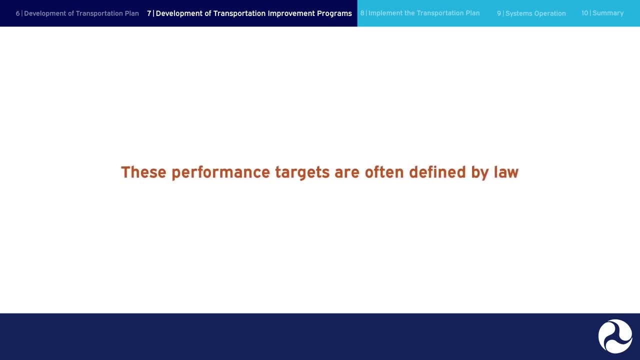 These performance targets are often defined by law and by their own regulations. For additional information about these laws and the relationship between TIP and STIP, please refer to the Transportation Planning Capacity Building Briefing Book. In practice example: As part of the TIP development process, the Plannersburg Public Works Department submits: 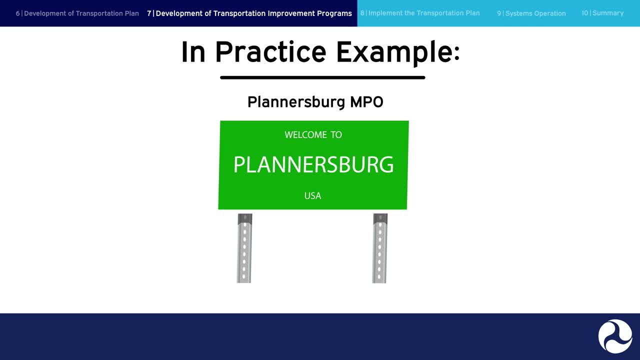 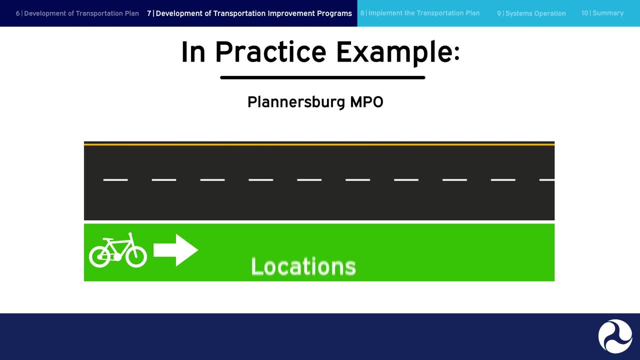 a proposal to implement one of the plan recommendations. located in their city, They develop a bike lane project proposal for consideration in the TIP that includes detailed information: locations, specifications, budgets, funding sources, timelines and cost estimates for environmental review, design and construction. 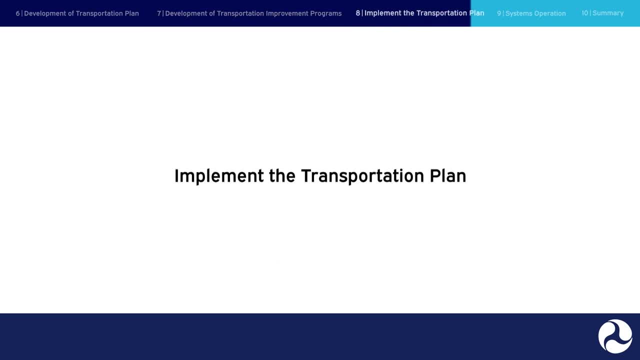 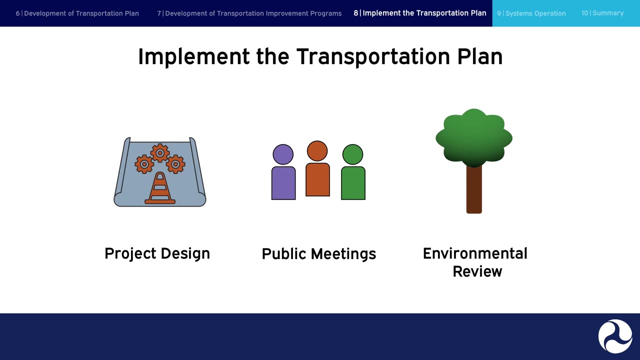 The permit Ganz as part, ofplease recommend for implementation. Implement the transportation plan. Projects recommended in the MTP are programmed in the TIP for funding and then moved toward implementation. Project design, public meetings and environmental review take place as the projec. 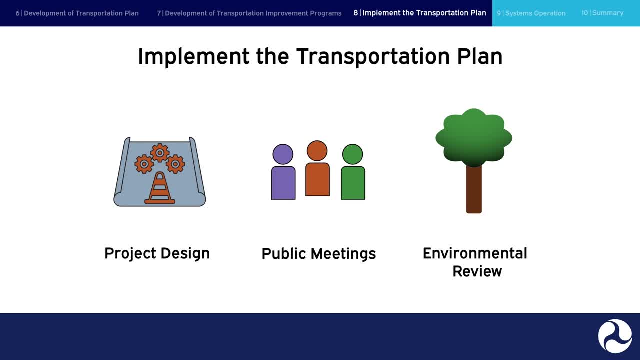 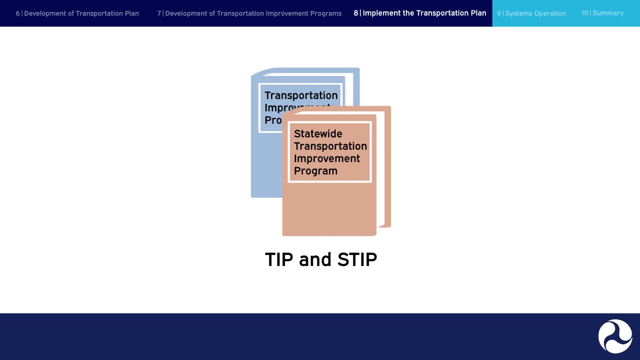 gains additional depth and detail in the development process. When the project and funding receive approval to be programmed in the TIP and STIP, the entity managing and building the project continues in the TIP. project can move forward towards preliminary engineering design, right-of-way and construction. 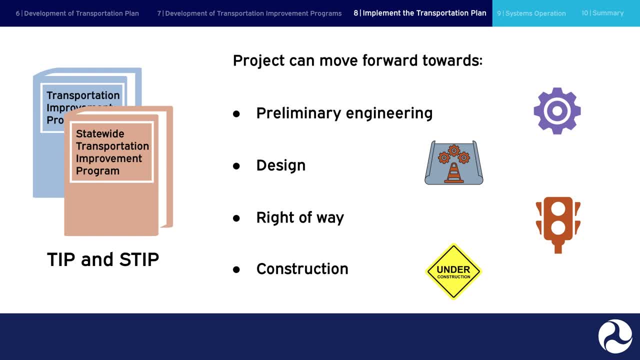 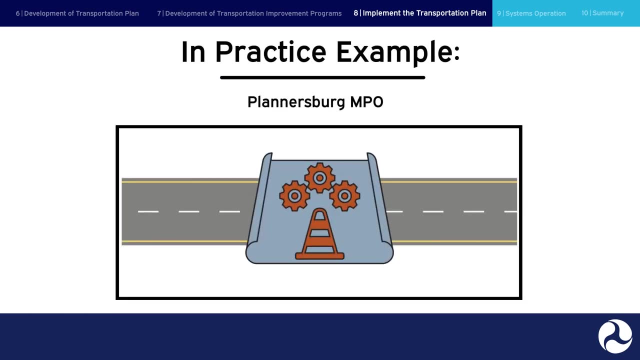 contracting and construction practices vary between states, organizations and municipalities, so you'll want to consult your agency's contracting and construction management guidelines for more information in practice. example: the project is included in the tip and the local public works department begins work to design and build the facility. 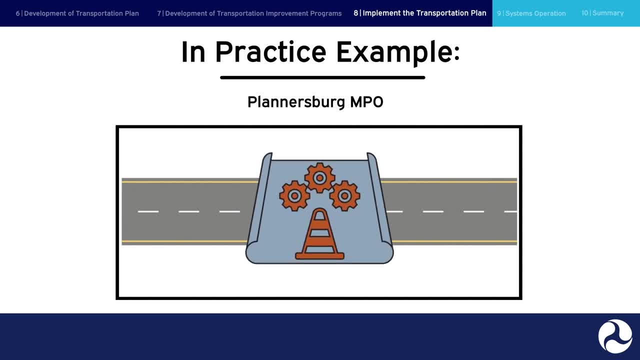 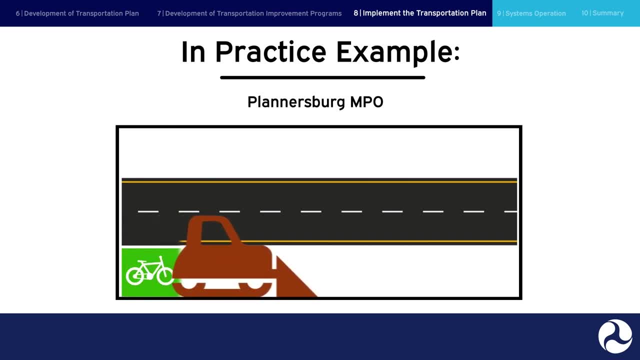 the city secures a landscape architecture and engineering consultant to move forward with designing the bike lane. during the design process, the city pursues environmental clearance and obtains required permits. once the design and environmental review are completed, the land necessary for the bike lane is purchased and the project is put out to bid. a contractor is selected.